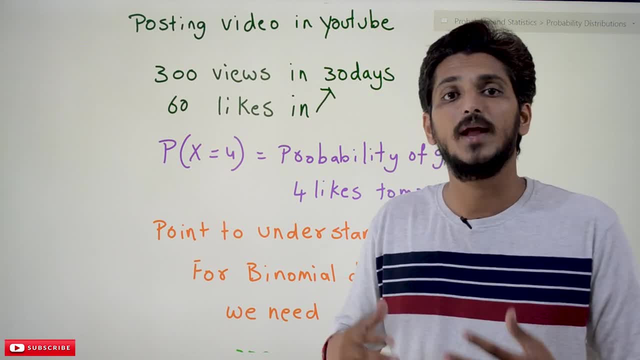 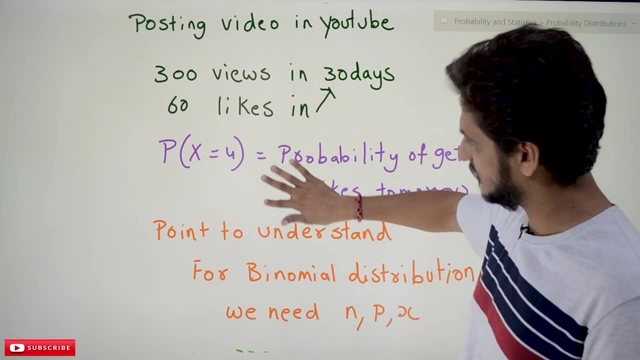 If N value, P value, X value is given, you can apply binomial distribution. Yes, this is what we have done in our last class. Yes, this is what we have done in our last class. So point to understand: for binomial distribution, we need N value, P value, X value. 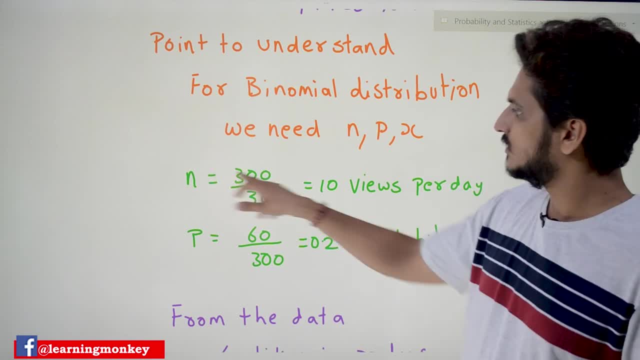 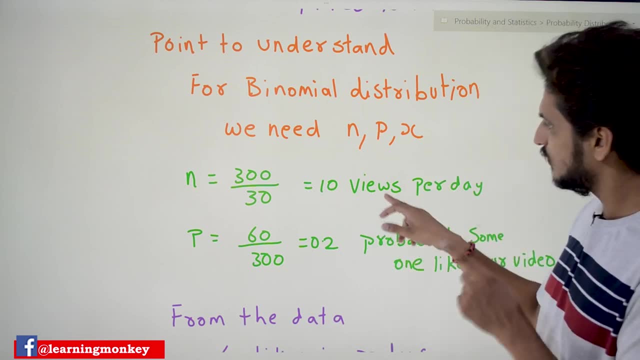 So how we identified the N value. So 300 views in 30 days. so N is equal to 300 by 30, that is equal to 10 views per day. So why we are doing it in 10 views per day? 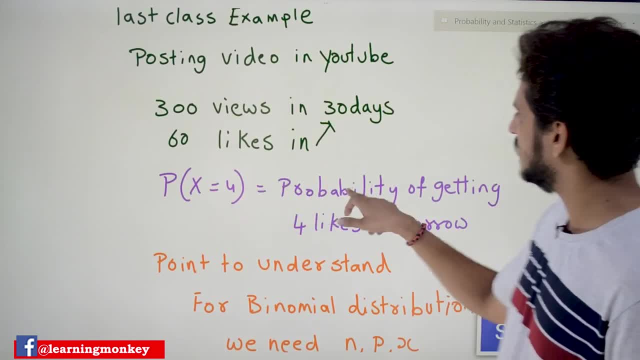 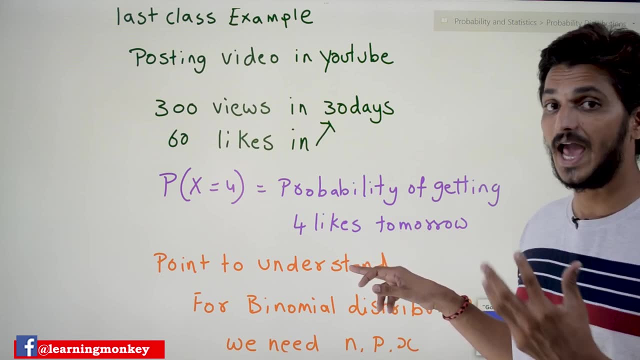 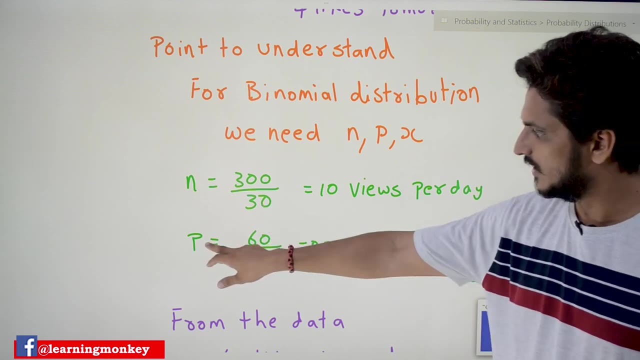 Because the question they are trying to ask is probability of getting 4 likes tomorrow. tomorrow means one day. That's why 300 by 30 in one day, what is the average views we are getting? That is what we are identifying. If 10 views happened in the next day, what is the probability of clicking like? button is 0.2. 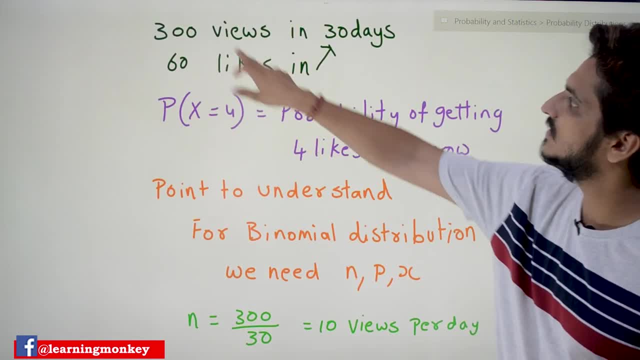 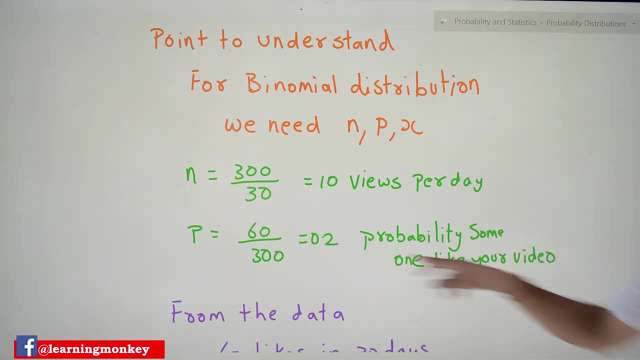 Probability is given by 60 likes in 300 views. That's why we got probability is 60 by 300. that is equal to 0.2. Probability. someone like your video is 0.2. 20% chance that they are going to like your video. 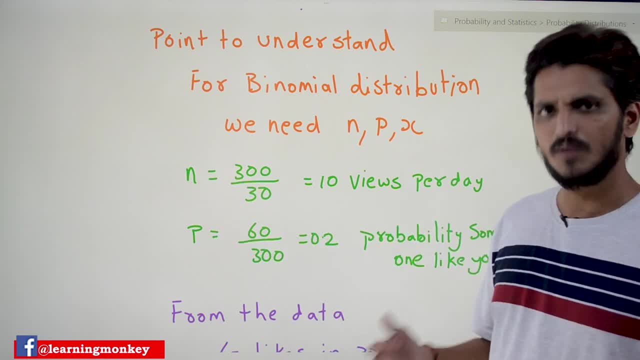 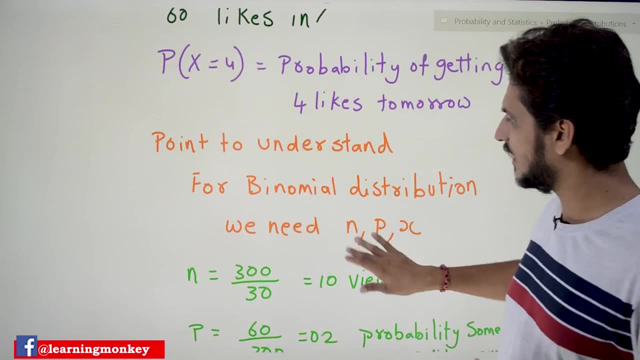 So, if N value is given, P value is given, we are applying binomial distribution And we identified the probability of X equal to 4.. This is what we have done in our last class, Coming to the point. this is the point you have to understand. 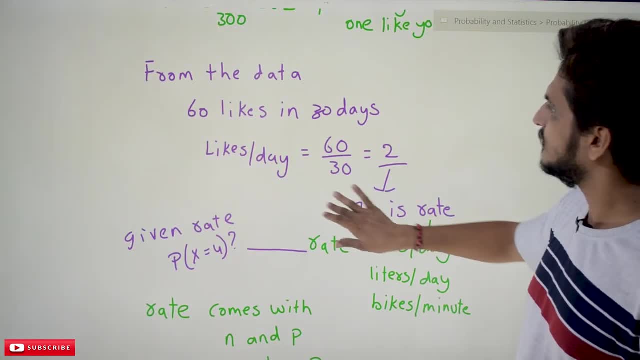 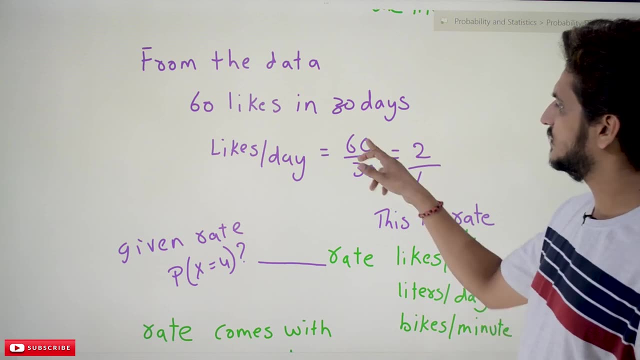 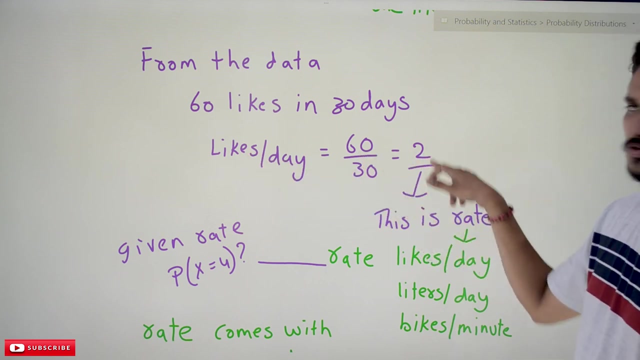 So from the data it was given that 60 likes in 30 days. If you convert this 60 by 30, that is equal to 2 likes per day. 2 likes per day. likes per day is given as 2.. 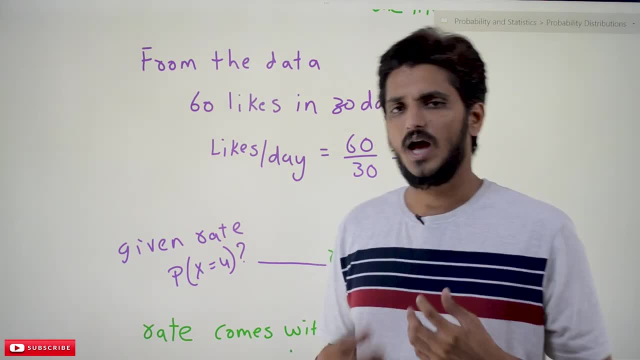 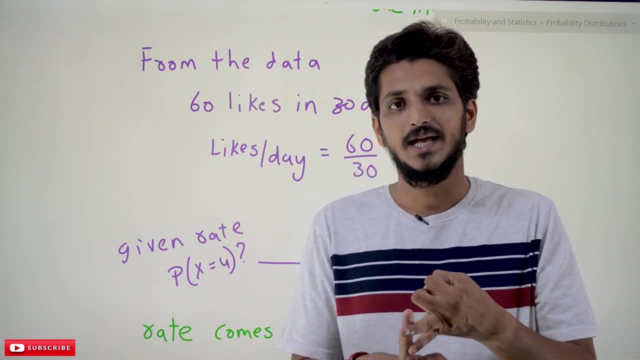 If someone has given you data, I am getting 2 likes per day. That is what they have mentioned. They didn't mention about N value. They didn't mention about P value. This is the case, which most of the situations happens in real time. 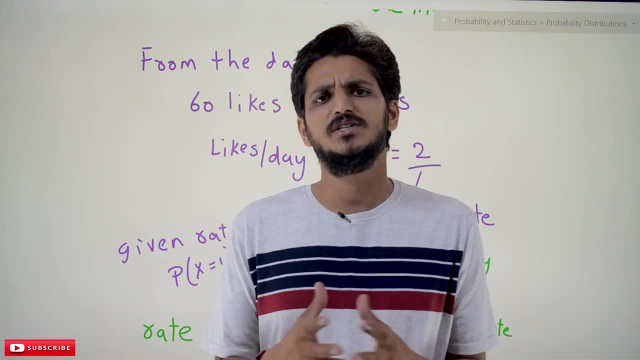 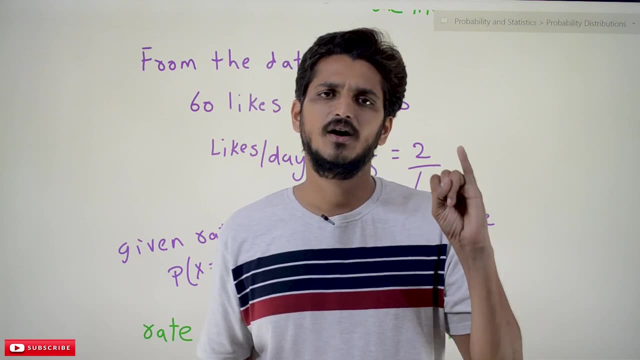 Because suppose, if you ask a doctor how many patients you will deal, how many heart patients you are going to deal in one day, What he says Every day, I will get 40 customers. In that we are having 30.. 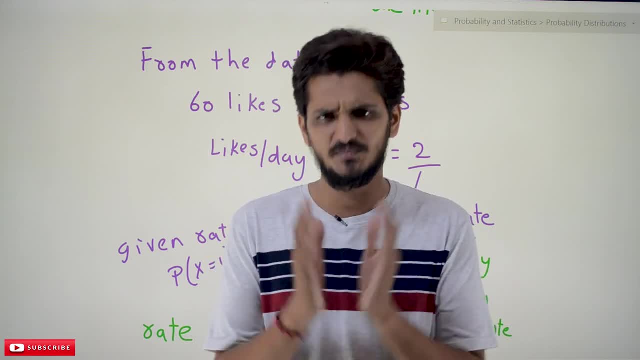 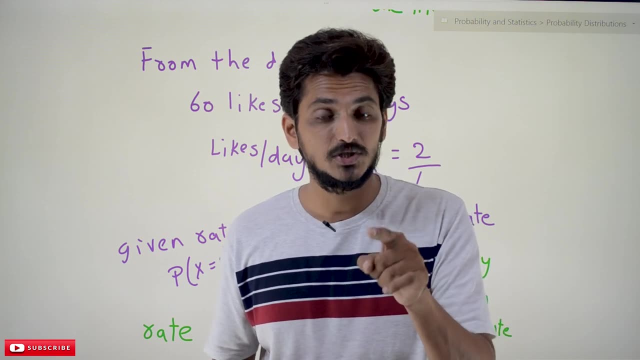 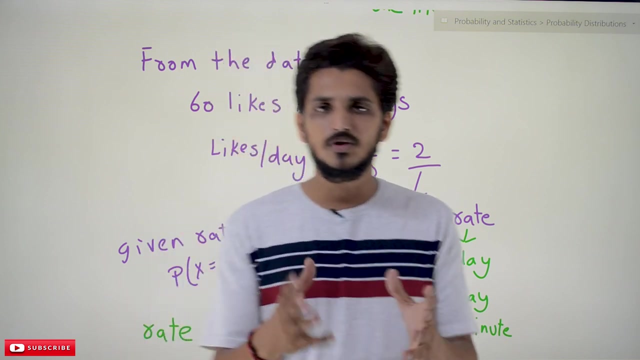 But 2 heart patients like that he will deal with. No, he simply says that on an average I will get 2 heart patients per day. In most of the real time situations, N value, P value is not available. Suppose if someone asks you to count number of bikes that are going in 1 minute on the highway. 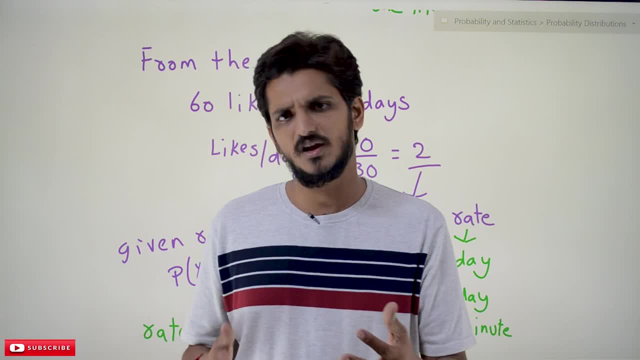 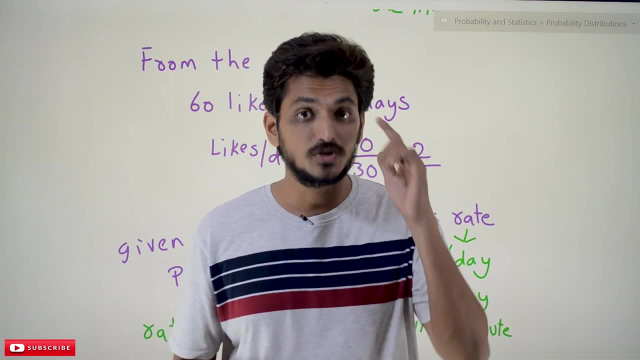 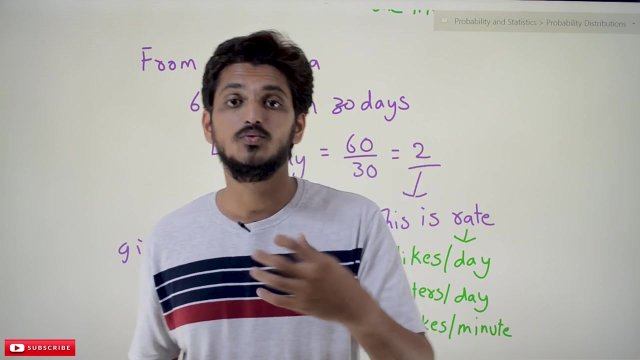 What you say. He keeps on counting the bikes and on an average you say that 10 bikes are going in 1 minute. So most of the times N value, P value, is not given by real time data. In that situations, what we have to do, that is what Poisson distribution is. 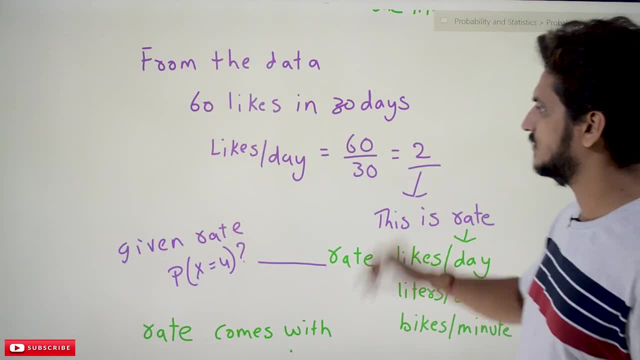 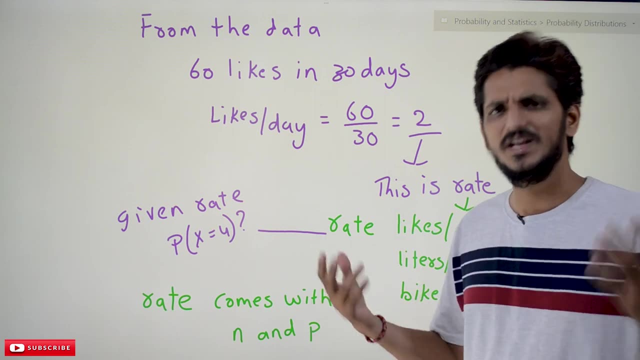 Let's try to understand when we are going to apply Poisson distribution. See if someone has given you likes per day. on an average, I am getting 2 likes per day. I don't care about how many views I got, and every day I just check the video. my likes are increasing. 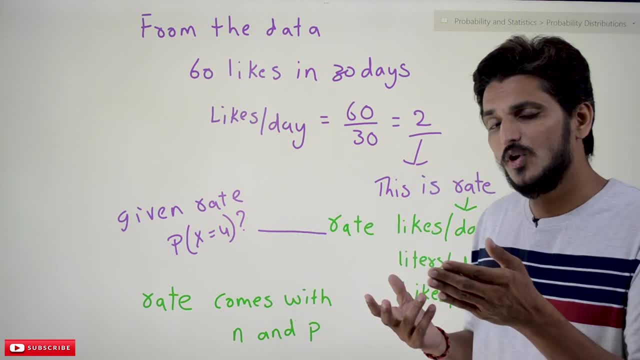 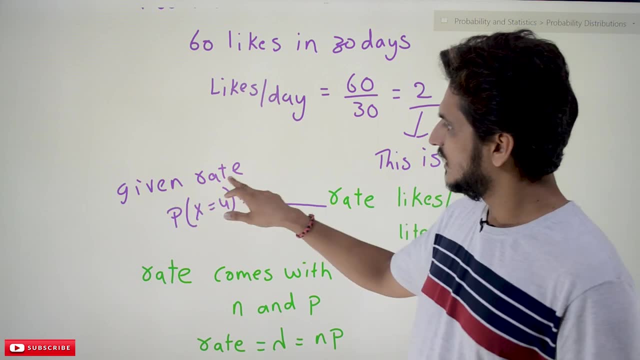 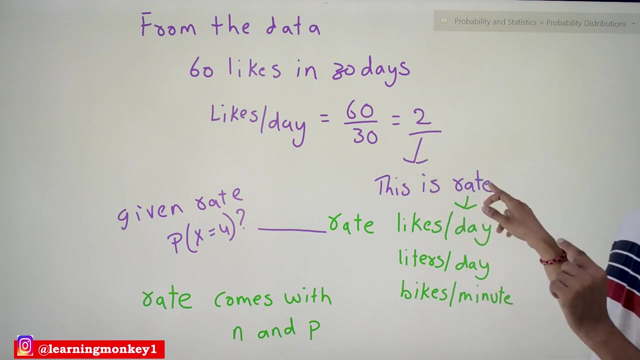 On an average- I had an idea about- On an average- I am going to get 2 likes per day. That is the information I have provided and I am trying to ask you Given see this- likes per day, 2 likes per day. this we call it, as this is called, rate value. 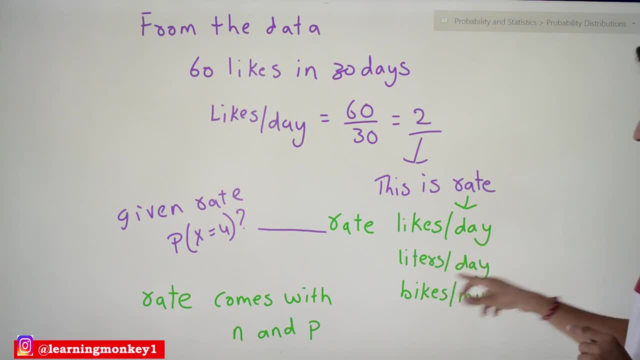 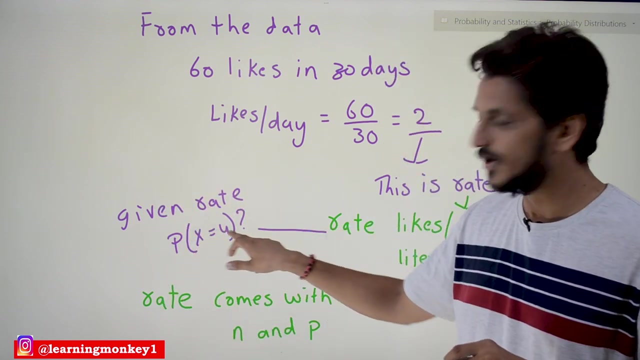 So likes per day, liters per day, bikes per minute- how many bikes that are going in 1 minute- All this comes under. we call it as rate value. If someone has provided you the rate value and they have asked you the probability that you are going to have 4 likes in our next day, 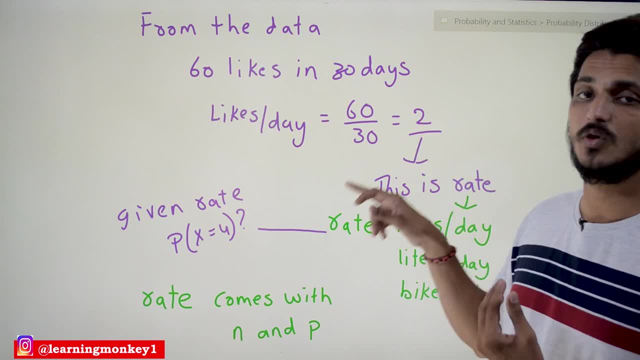 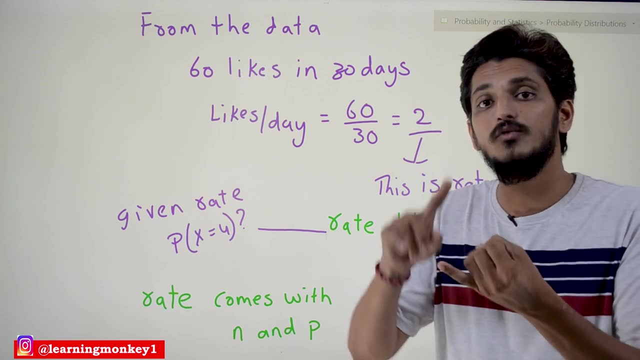 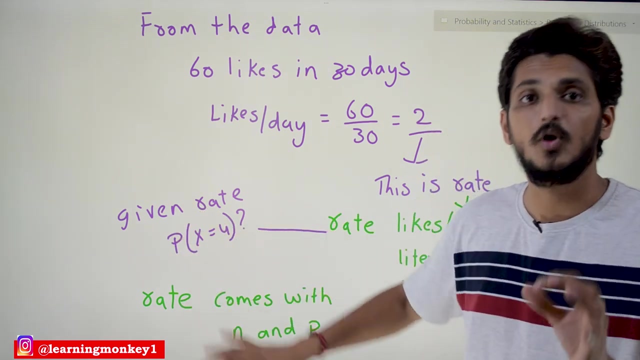 They have given? on an average, you are getting 2 likes per day. What is the probability you are going to get 4 likes in our next day? Without having N value, without having P value, you can identify this probability value using Poisson distribution. 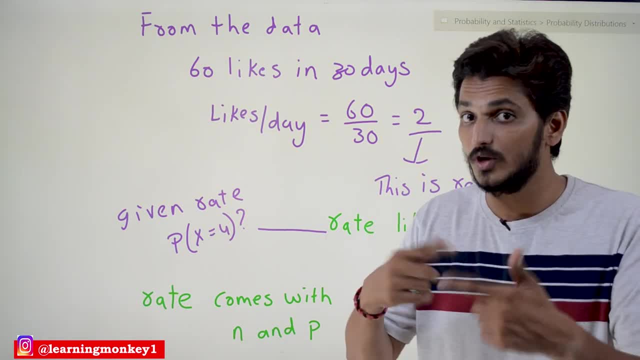 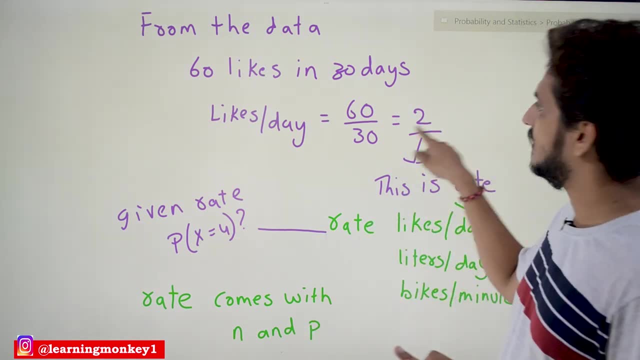 So we are going to apply Poisson distribution. When we are going to apply Poisson distribution If N value is not there and P value is not there? someone has given you the rate value Likes per day, liters per day, bikes per minute. this we call it as rate value. 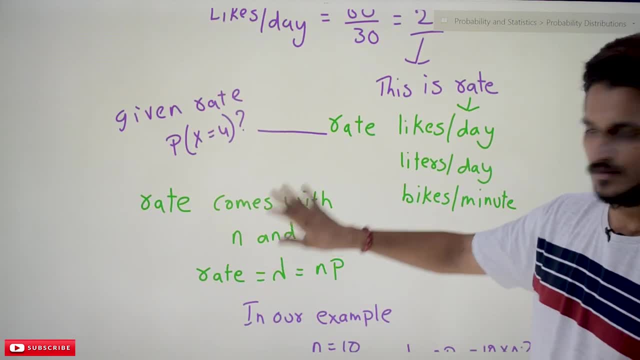 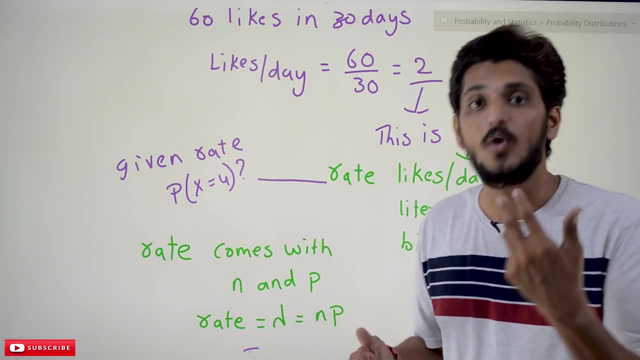 This we consider it as rate comes with. so this we consider it as lambda. Lambda means rate has been given. Then we are going to apply Poisson distribution. So in the mathematical sense we are going to apply Poisson distribution. 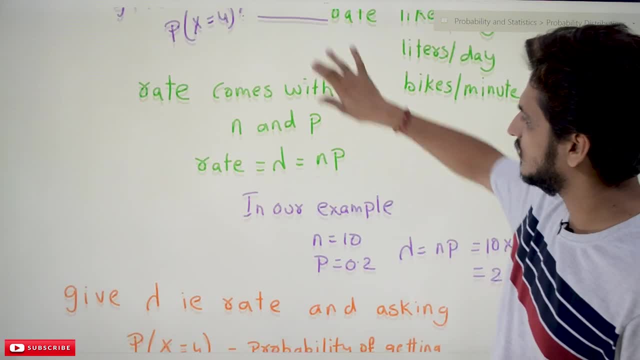 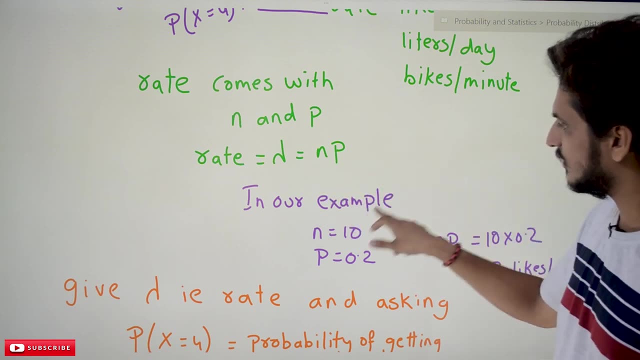 So in the mathematical sense we need to understand one more concept also. Rate is equal to lambda is equal to Np. See in our example: N is given that 10 views per day and P is given that 0.2.. 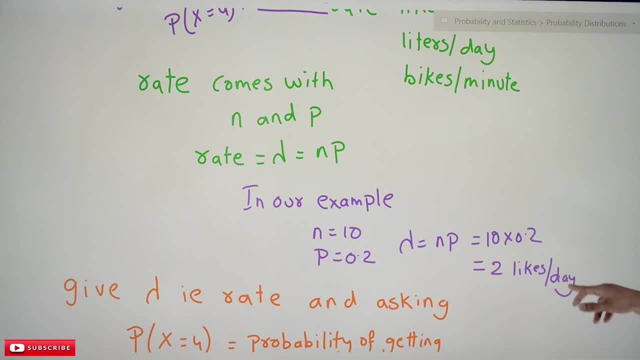 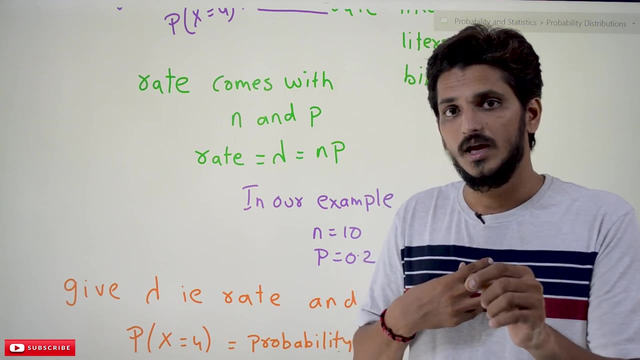 Np is 10 multiplied by 0.2, that is 2 likes per day. So indirectly, when they have given you the rate value means what we have to understand: Multiplication of N value And P value, we are getting it as rate value. 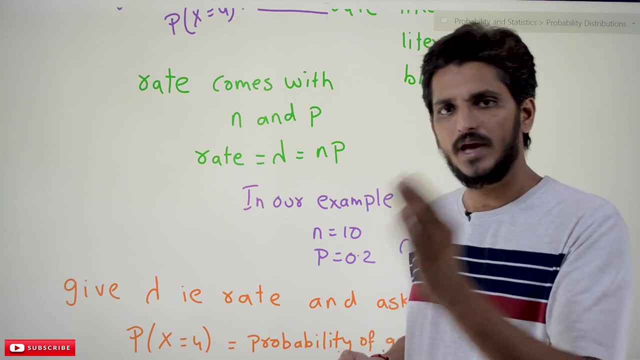 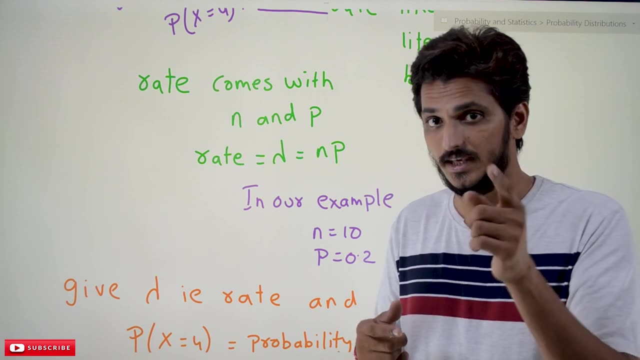 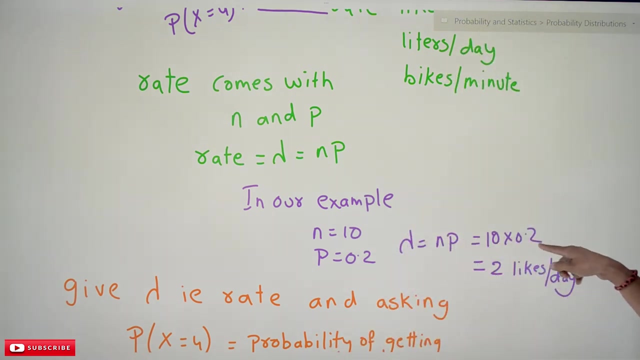 That is the point you have to understand. If someone says you 10 bikes are coming in one day Indirectly, they have provided you the data N multiplied by P. So that's why you got that. lambda is equal to Np, that is, 10 multiplied by 0.2. that is equal to 2 likes per day. 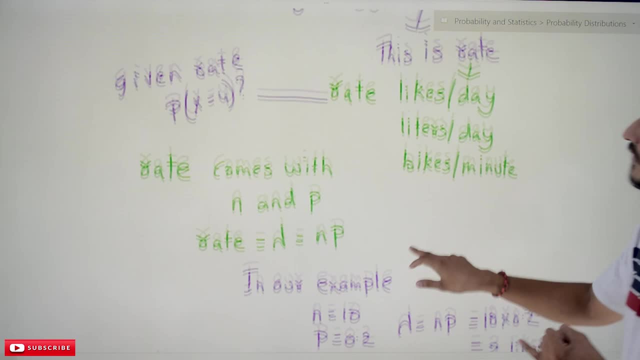 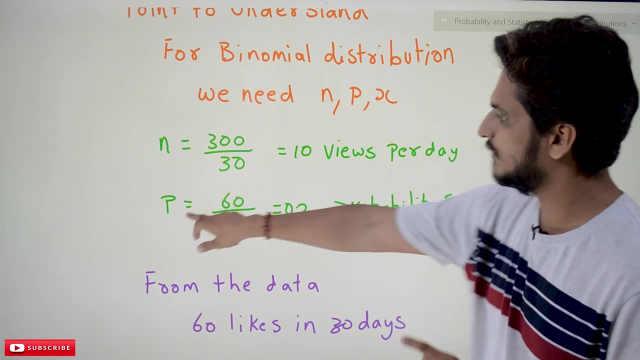 This data, 10, N is equal to 10, P is equal to 0.2. come from our previous data: N is equal to 0.2.. N multiplied by 2, N multiplied by P, that is 10 multiplied by 0.2, which we call it as 2 likes per day. 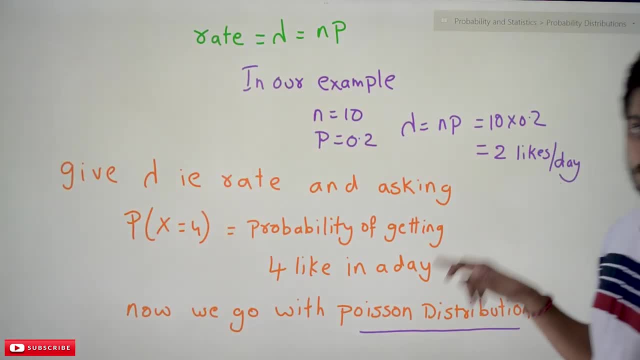 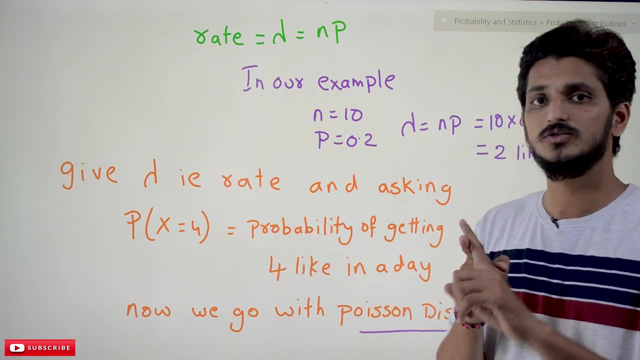 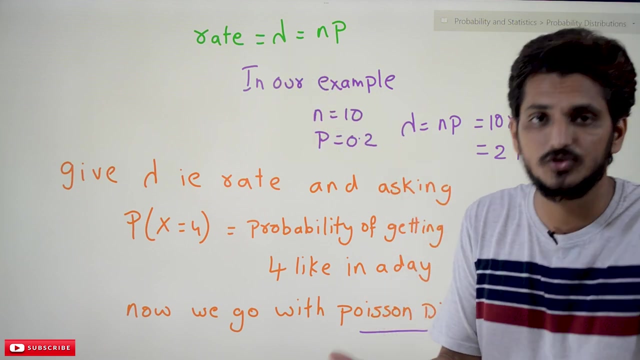 We got this information, rate value. So that is the point you have to understand. If someone has given you but you don't know the N value and P value, Multiplication of both the values, you got it as lambda. If someone has provided you the lambda value means rate value, you can apply Poisson distribution. 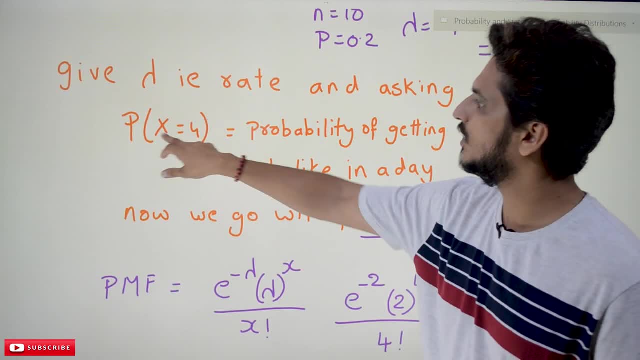 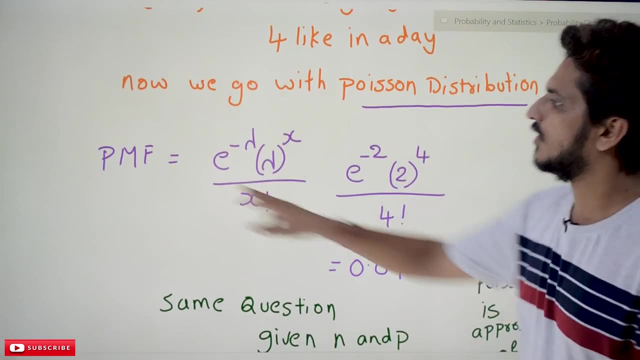 So given lambda, that is rate and asking probability of X is equal to 4. Probability of getting 4 likes in a day. Now we go to Poisson distribution: Probability. mass function for Poisson distribution is e power minus lambda. lambda power X by X factorial. 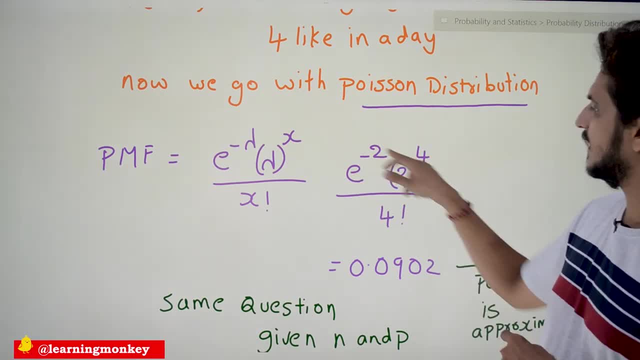 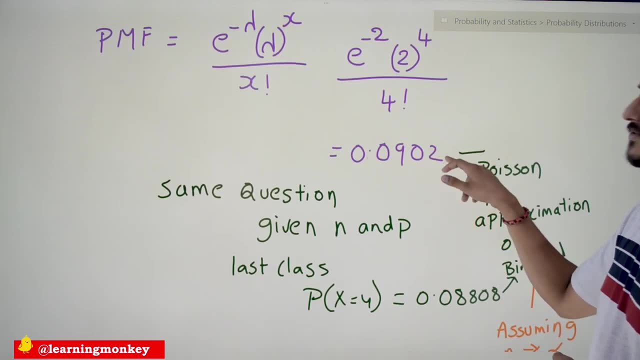 When you substitute e power, lambda is 2.. e power minus 2, 2 power: 4.. X is 4.. 4 likes per day divided by 4 factorial, You got the value 0.0902.. The same data you applied in our last class example with N value and P value in binomial distribution. 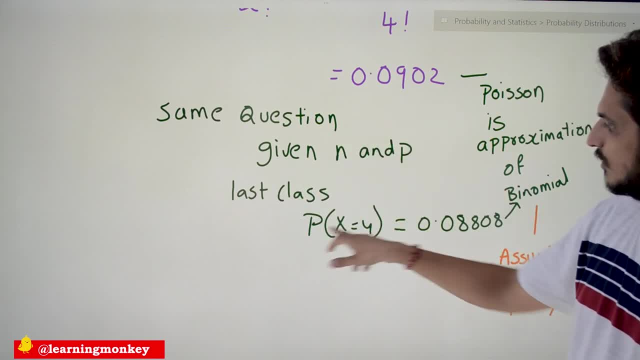 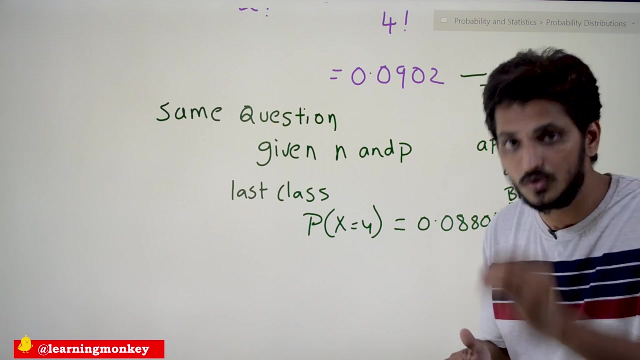 So when you substitute N value, P value in binomial distribution and probability of X is equal to 4, which we got it as 0.08808.. It approximately near to the Poisson distribution value. That's why we say it as a Poisson distribution is an approximation to binomial distribution. 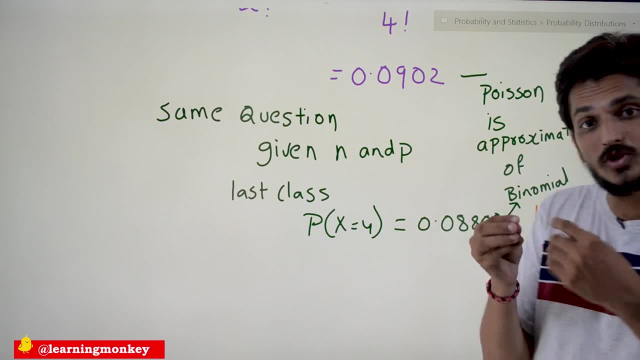 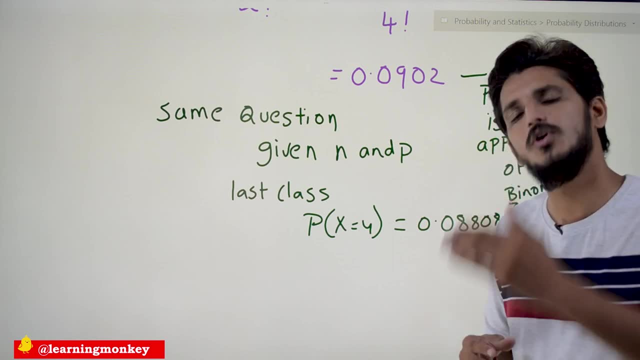 We didn't get exactly the same, but almost all near to the same probability values you will get. So Poisson distribution is an approximation to binomial distribution. When we are going to apply binomial, when we are going to apply Poisson distribution, 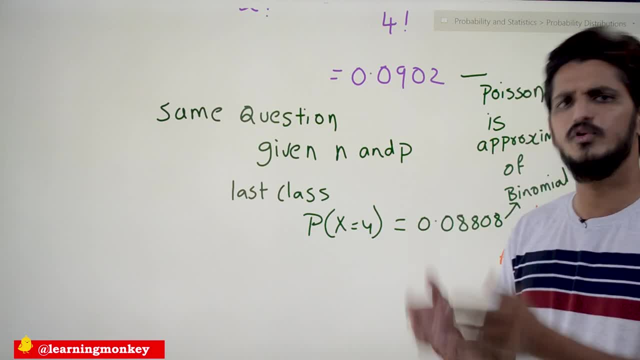 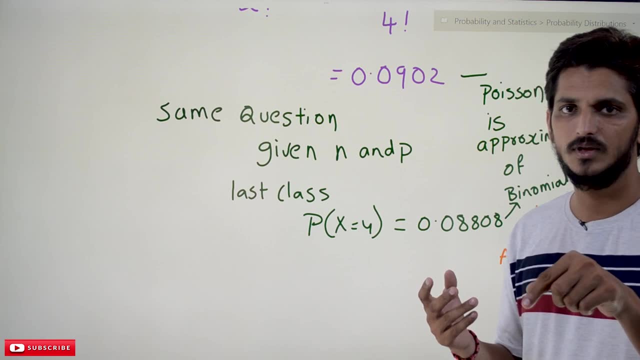 If someone has given you the N value and P value, go with binomial. If they have most of the time they are going to give you the rate value means lambda value. Then go with Poisson distribution. Both are giving you the same, approximately same Poisson distribution. 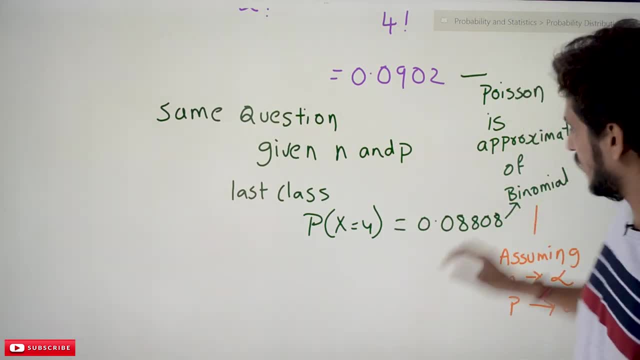 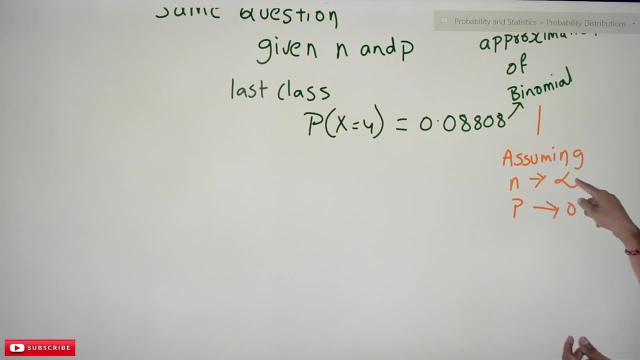 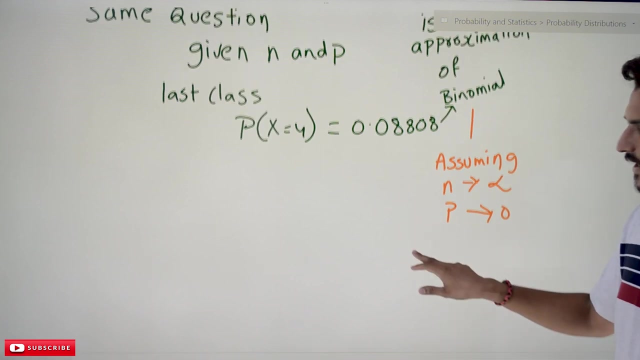 The same probability values. And one more important point you have to understand: We don't know the N value and P value. So we are assuming that N is almost near to infinite And P is almost near to zero value. And in our coming classes we are going to understand why we assume that N is almost near to infinite value. 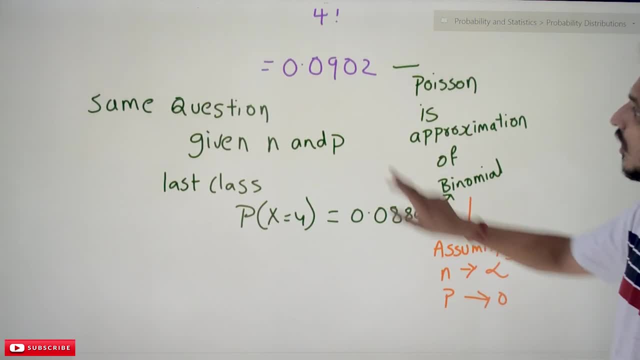 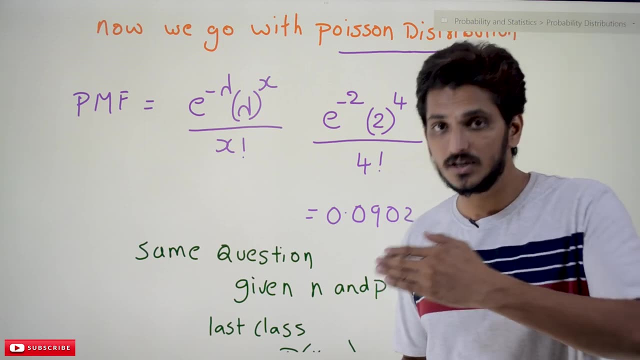 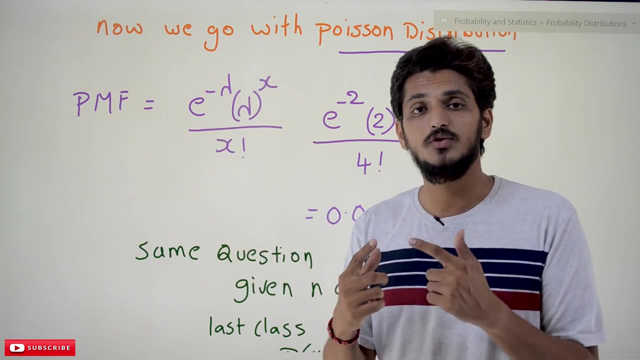 And why P is almost near to zero value And how we got this probability mass function. Assuming that N is equal to infinite and P is almost near to, approximately near to zero, We got this probability mass function, How we got this. These points you are going to understand in our coming classes. 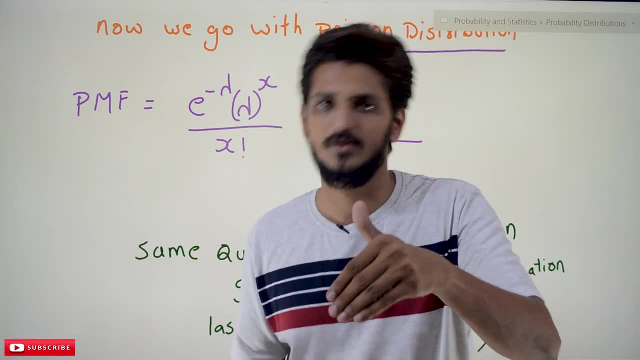 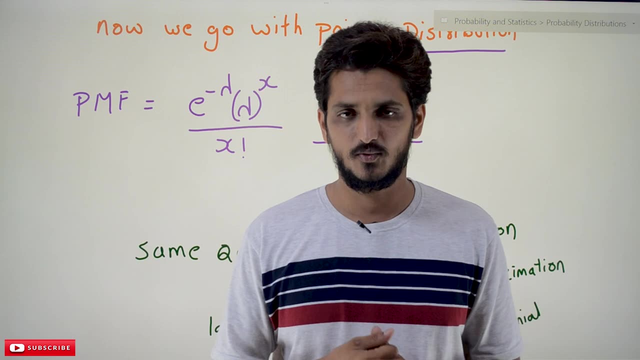 This class we concentrated on when we need to apply Poisson distribution. Hope you understand the concept. If you have any questions regarding the concept, Please post your questions in the comment section below. Thanks for watching. If you haven't subscribed to our channel, please subscribe to our channel. 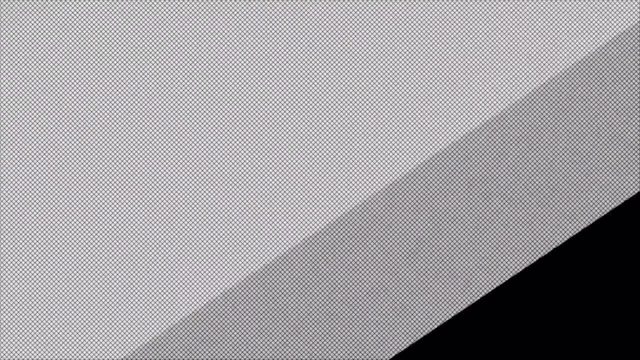 And press bell icon for the latest updates. Thank you, See you in the next video.